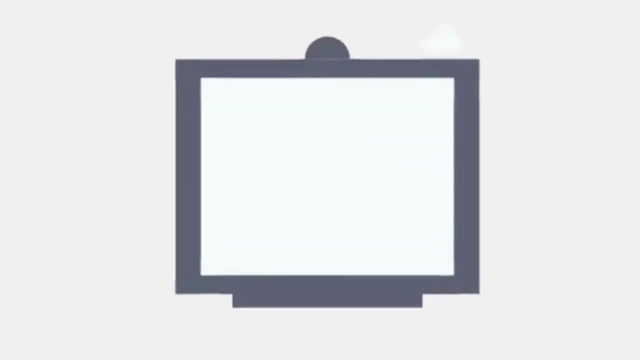 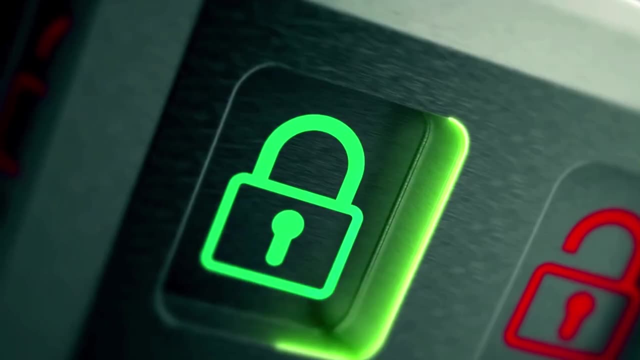 This is especially important for websites that handle sensitive information, such as online stores and banking websites. When a website has a valid SSL certificate, it displays a padlock icon in the address bar of the browser, which can help to increase user trust in the website. 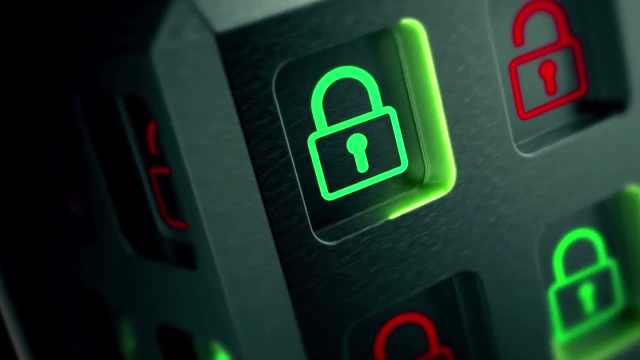 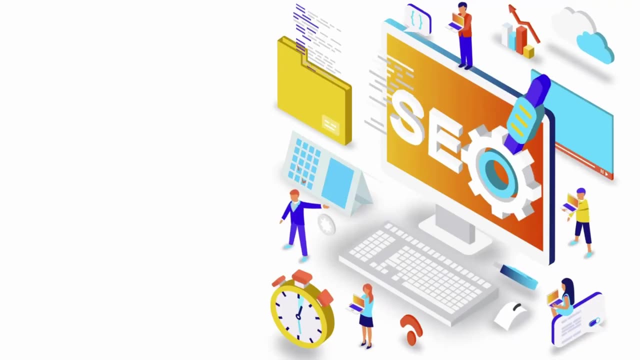 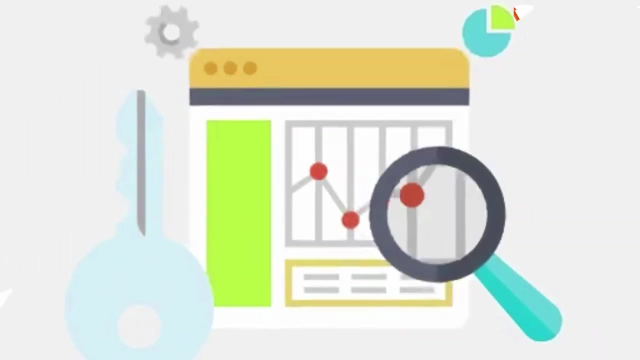 This is especially important for websites that handle financial transactions or sensitive personal information. SEO search engines such as Google consider the use of SSL as a ranking factor when determining the relevance and credibility of a website. As a result, having an SSL certificate can help to improve a website's search engine rankings. 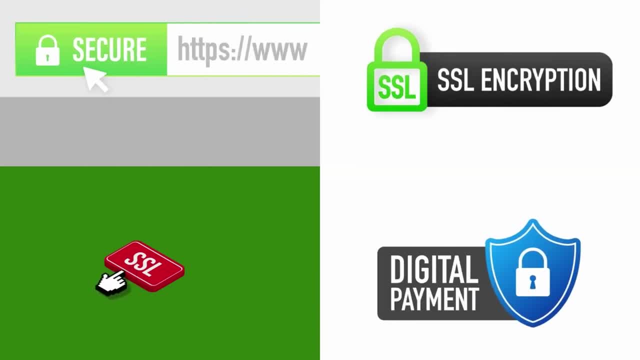 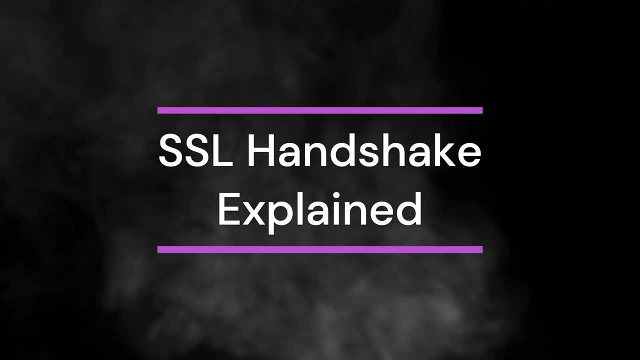 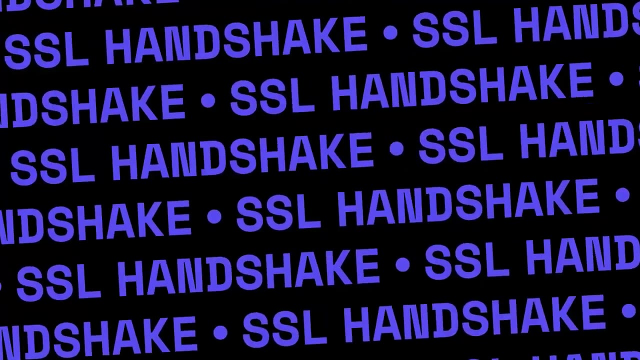 In summary, SSL is important for websites because it helps to secure sensitive information, increase user trust and improve search engine rankings. How to use SSL Handshake. SSL Handshake will negotiate the encryption and authentication methods that will be used to secure the connection. 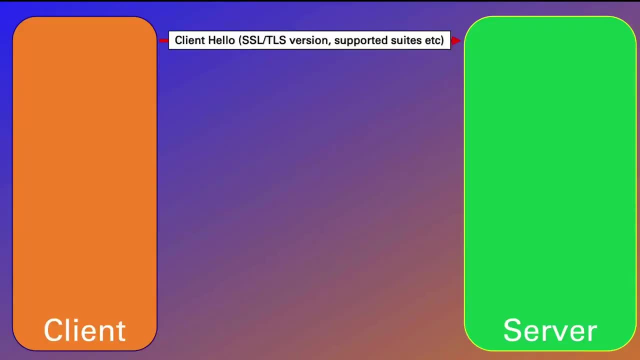 SSL Handshake consists of several steps: 1. The client sends a client hello message to the server which includes information about the client's SSL TLS version and a list of supported cipher suites indicating the encryption and authentication methods. 2. The server responds with a server hello message of its own which includes its own. 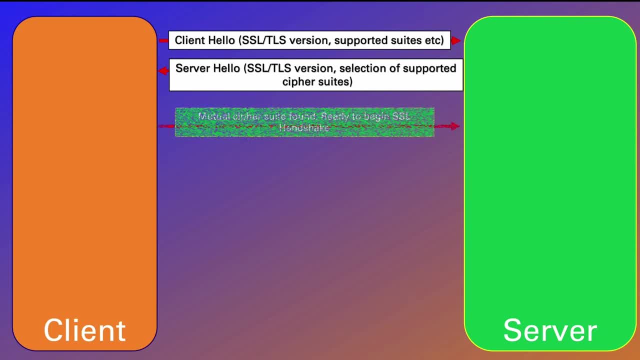 TLS version and a selection of cipher suites that it supports. 3. The client and server use this information to negotiate a mutually supported cipher suite. If a mutually supported cipher suite is found, the client sends a message to the server indicating that it wants to begin the SSL handshake. 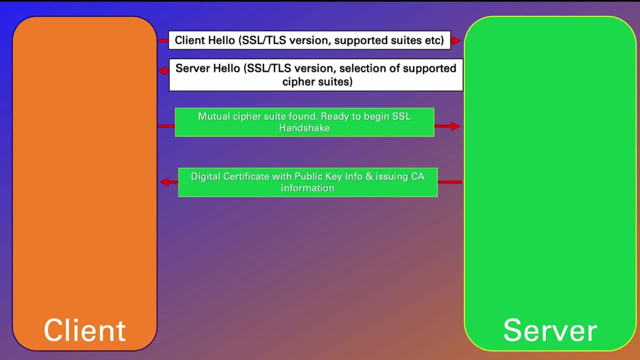 4. The server responds with a message containing its digital certificate, which includes its public key and information about the issuing certificate authority. 5. The client verifies the authenticity of the certificate using the CA's public key, which is stored in the client's device or browser. 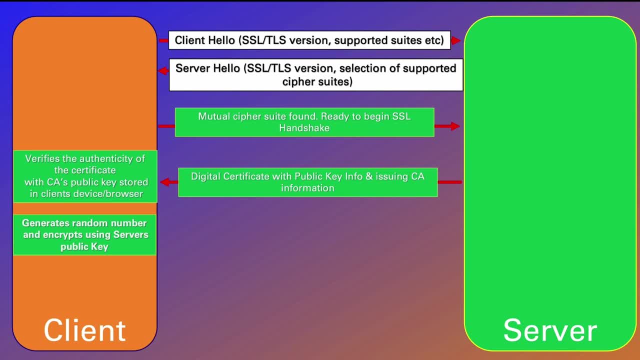 6. The client generates a random number and encrypts it using the server's public key. 7. It sends this encrypted number, known as the pre-master secret, to the server. 8. The server uses its private key to decrypt the pre-master secret and generates a session. 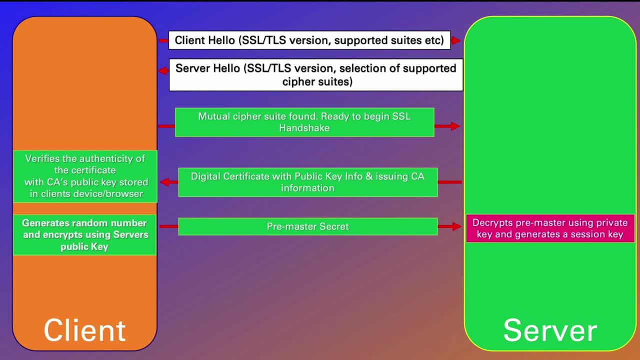 key that will be used to encrypt and decrypt data during the SSL session. 9. The server sends a message to the client with the master secret or the session key that will be used for transmitting data. 10. Both client and server sends client and server-finished messages.